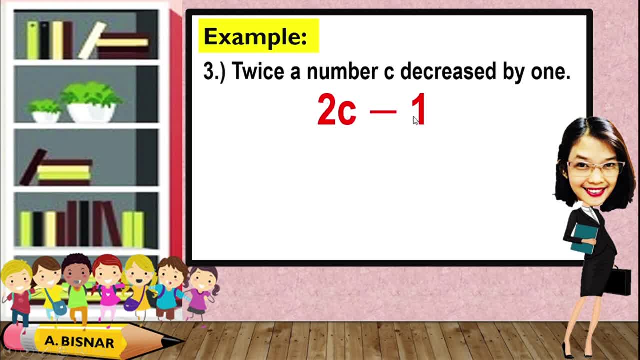 written as 2 C minus 1. again, it is a combination of numbers and variables and the present operation in here is subtraction and in here there is a multiplication. next, the cube of Y divided by 9, which can be written as Y cube over 9. and again, this is an example of an algebraic expression because it is: 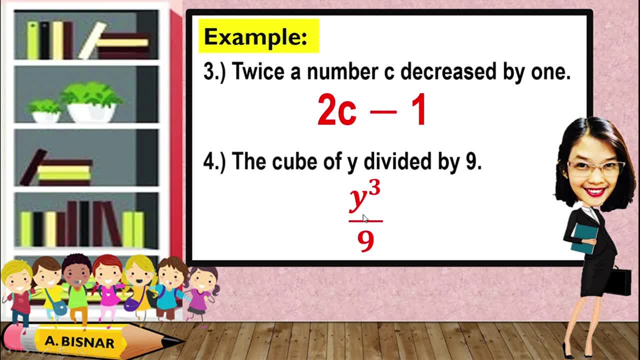 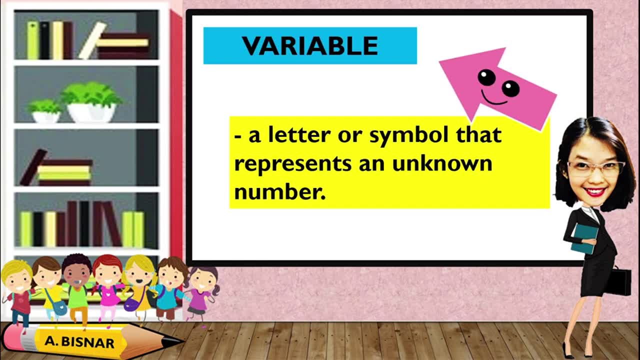 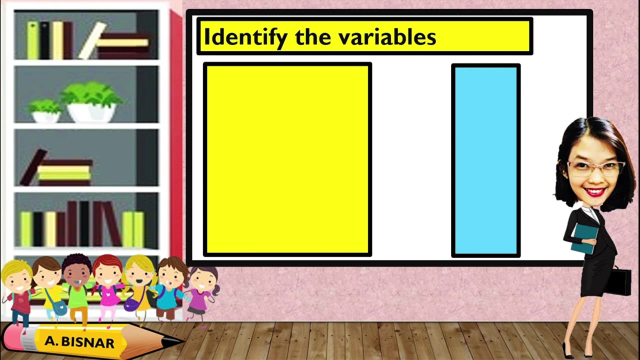 again a combination of number and variable, and the present operation in here is division. so let us now define a variable. a variable is a letter or symbol that represents an unknown number, so let us have this as our example. let us identify the variables for number 1, 3a plus 2 from: 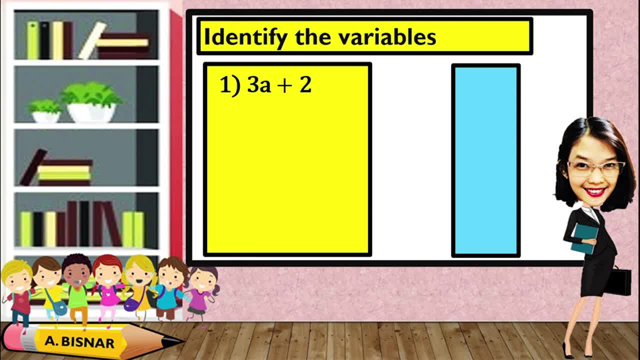 the given definition. again, it is a letter or a symbol that represents an unknown value, which means that a variable is a letter or symbol that represents an unknown value, which means that the variable in here is a another 7 B minus 4 C. so the variables in here will: 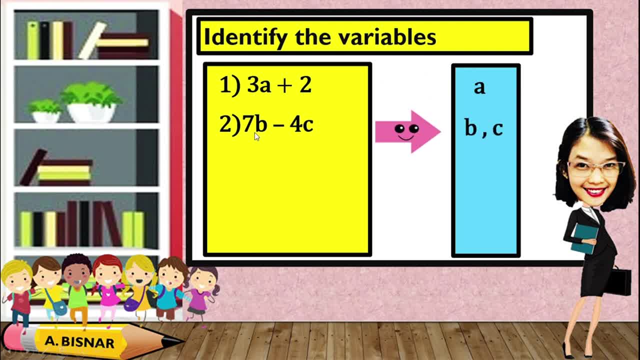 be B and C, B and C, another 6, x, y, Z. so what could be the variables? that's correct. the variable is a another 7b minus 4 C, so the variables in here will be b and c, another 6, x, y, z. so what could be the variables? that's? 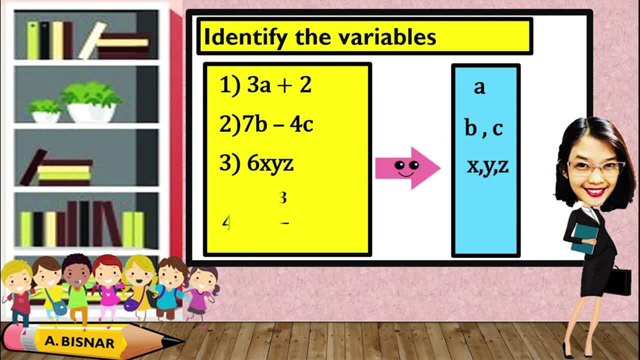 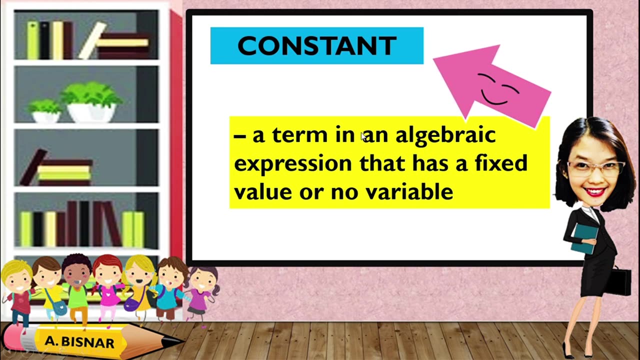 will be X, Y and Z. and for the last one, say we have M cubed over 9. now what could be the variable? that's correct. the variable will be M. it's very easy, right? so let us now identify what is the constant. a constant is the term in: 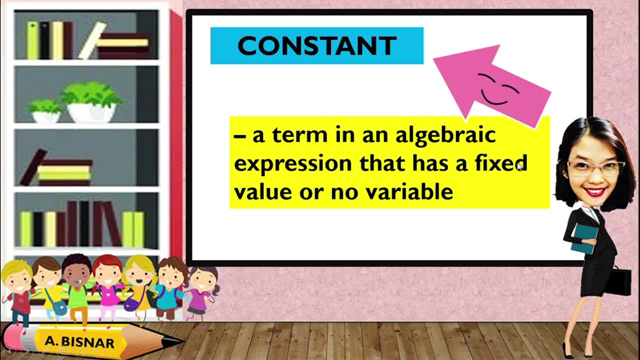 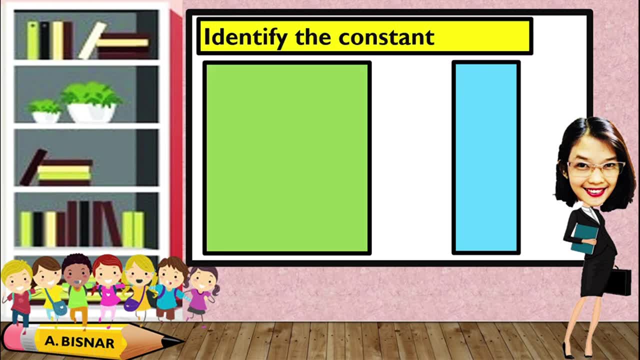 algebraic expression that has a fixed value or no variable. so let us have this as our example from the given direction. we need to identify the constant. say we have 3 a plus 2. again, it has a fixed value or it has no variable. in here: 3 a. 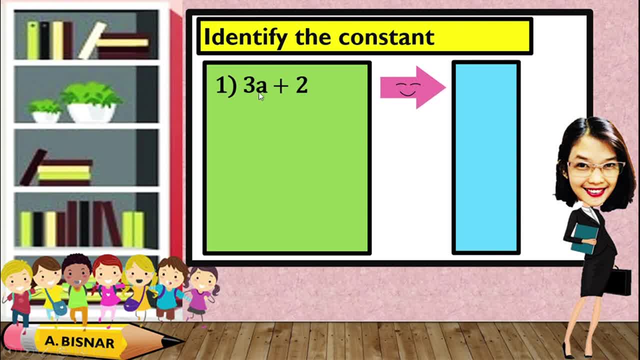 there is an unknown value which means this is a fixed value or it has no variable. in here, 3 a, there is an unknown value which means this is not fixed, and therefore this means that 2 is the constant, another 7 B minus 4 C. 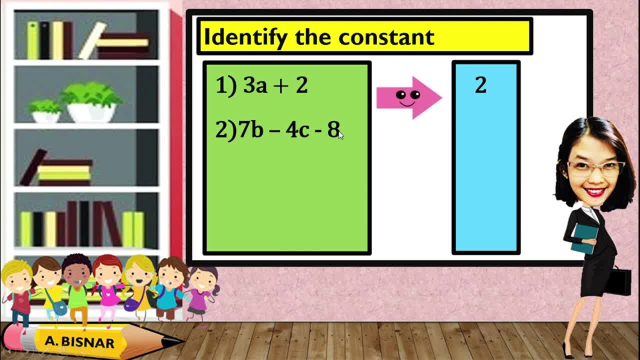 minus 8. now what could be the constant? again, it must have a fixed value or no variable. that's correct. and the answer is negative: 8. another X squared plus 4. now what could be the constant? that's correct. the answer is 4. and for the last one, 5 B minus 2 Q. now what could be the constant? 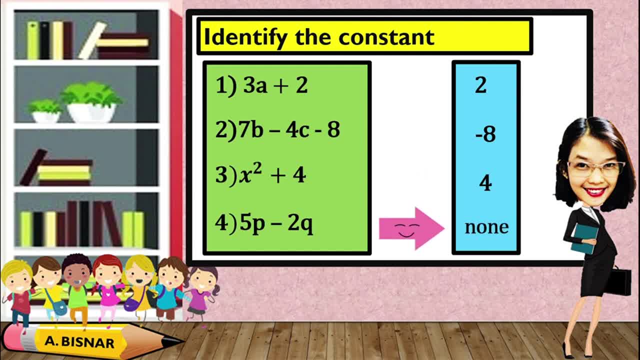 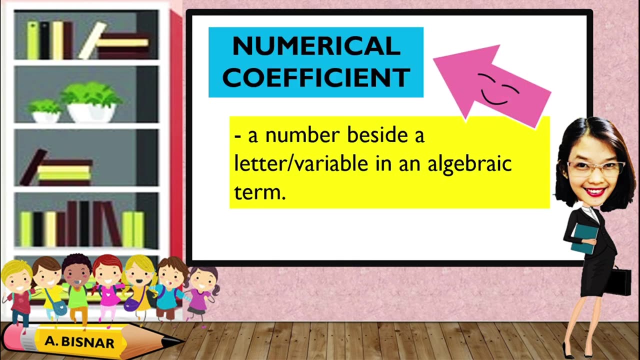 that's correct. none, because there is no constant in this algebraic expression, because there are variables in here which are a known value, which means this: two terms are not fixed. next let's identify numerical coefficient. a numerical coefficient is a number beside a letter or a variable in an algebraic term, while literal 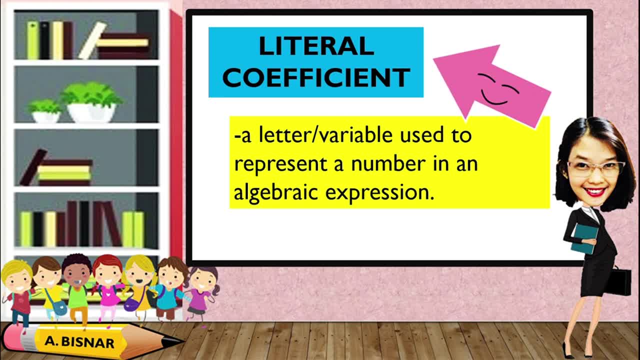 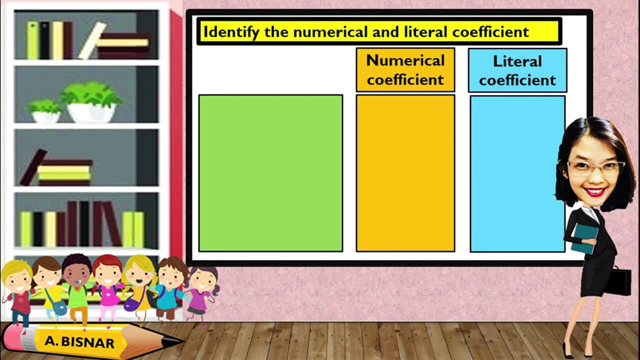 coefficient is a letter or a variable used to represent a number in algebraic expression. so let us have this as our example. we will identify the numerical and the literal coefficient for number one 3a. the numerical coefficient will be true and the literal coefficient will be a. it's very easy, right. we just need to. 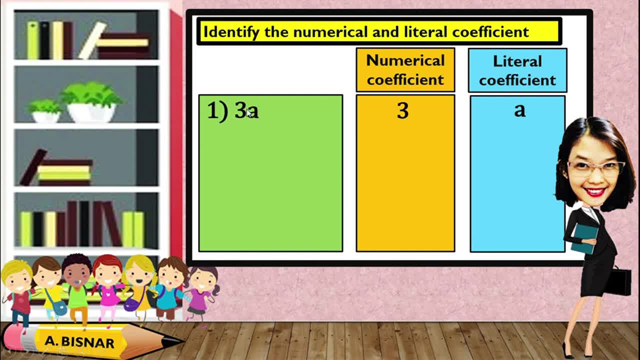 identify, make sure of these numbers and these numbers according to the classical, the number and the letter. the number will be the numerical coefficient and the letter will be the literal coefficient for number 2 B minus 4 C. well, I think your answer is just 4. however, in here we have B. this means